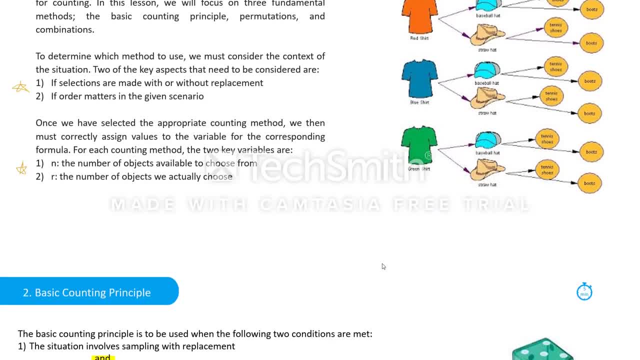 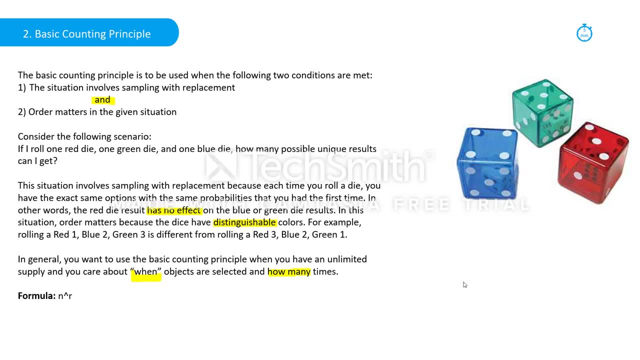 So one type of method that can be used is the basic counting principle, And we want to use this if it's a situation that has sampling without replacement and if order matters in that situation And if that is the method we want to use. the formula is going to be n to the r. 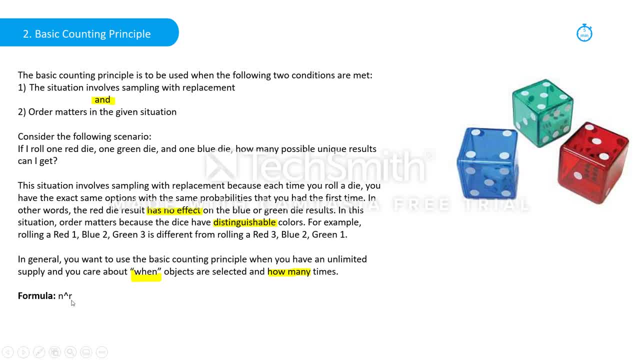 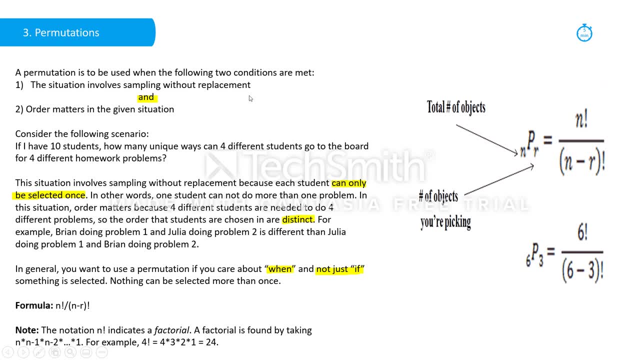 The options available to the number of options we actually choose. Another method we could use is a permutation, And this is a situation that involves sampling without replacement, So a choice cannot be chosen again And order matters in that situation, And, as we can see over here to the right, this is the formula for a permutation. 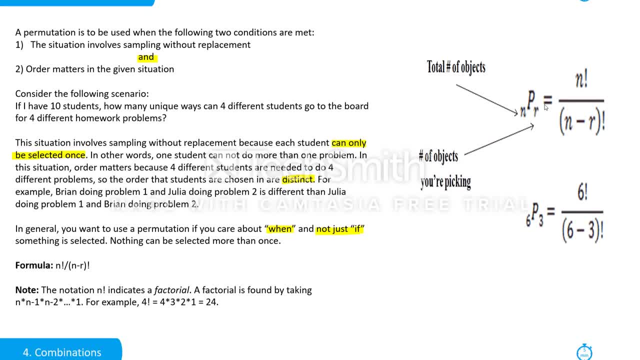 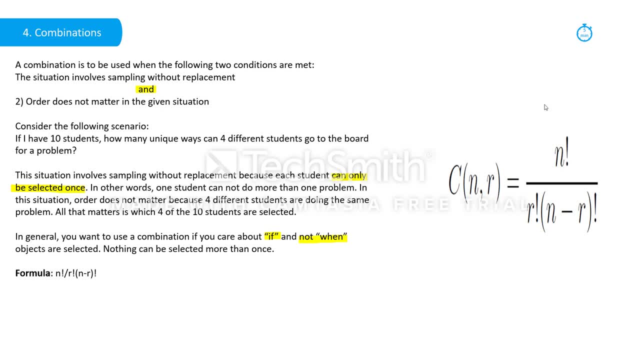 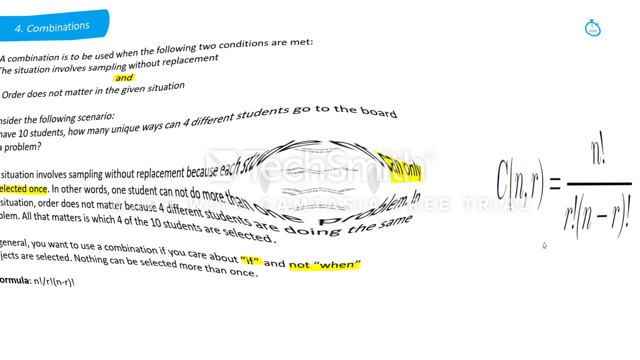 n factorial over n minus r factorial. And the other type of method we might choose is a combination, And this is a situation that involves sampling without replacement And order does not matter. And this is our formula for a combination: n factorial over r factorial times n minus r factorial. 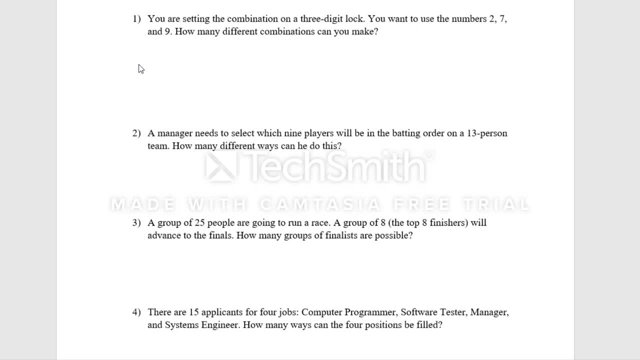 Now I want to step you through a couple example problems that involve combinatorics. So number one: we might be tempted to say it's a combination right away, because the word combination is in the problem. But if we look a little deeper we actually find out that this is a permutation. 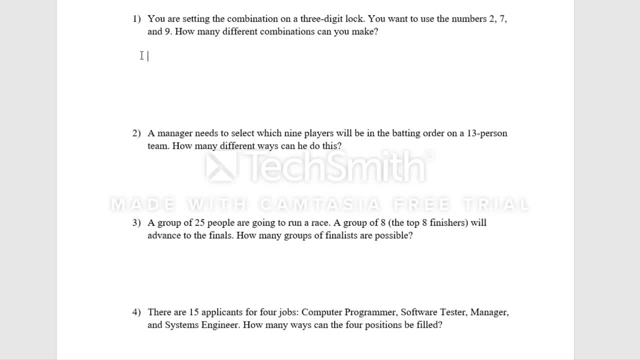 So the first thing we do is determine if this problem uses replacement or not. And in this problem we will see that there is no replacement, Because we want to determine how many different combinations there are. So once let's say 2,, 7,, 9 is one of our combinations. 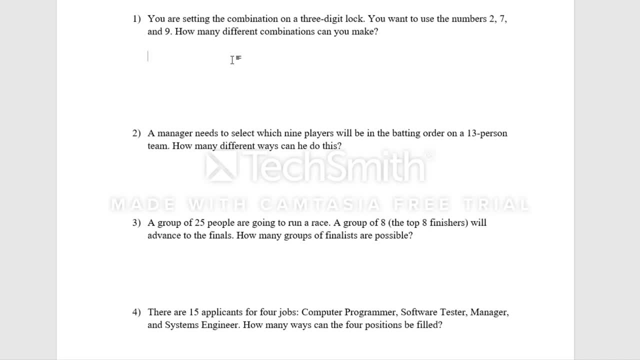 Well, we're trying to come up with a unique combination, So 2,, 7,, 9 could not be selected again. So we know that there's no replacement in this problem. Next thing we look at is whether order matters or not. 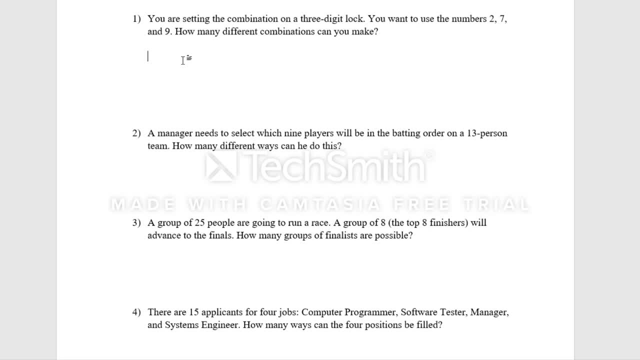 In this problem, order does matter, Because 2, 7, 9 is certainly different than 9, 7, 2.. So we know that this is a permutation, Because order matters And there's no replacement. The next thing we do is figure out how many options are available. 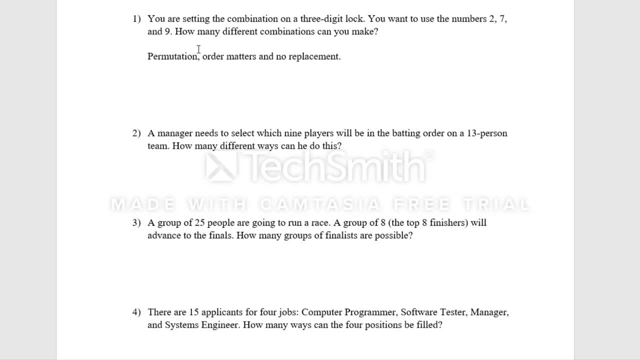 and how many things we actually choose. So from the problem we know that we only have 3 options available: 2,, 7, and 9.. So n is 3.. And then the number of things we're actually choosing is 3 as well. 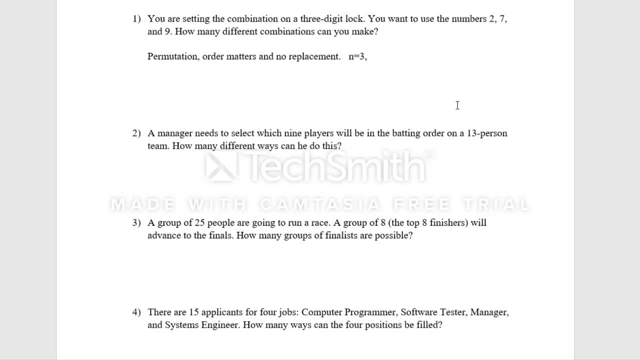 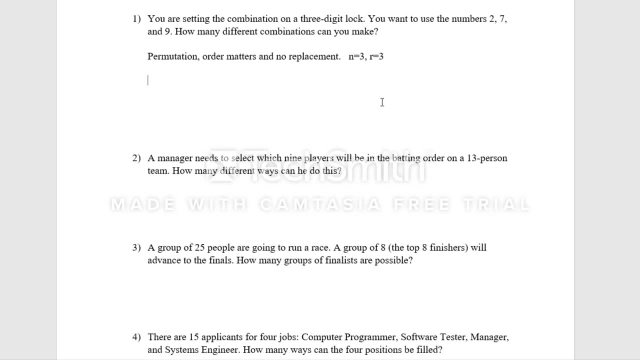 Because we are setting 3 digit locks, So we're going to choose 3 of those available numbers. So our formula here is n factorial over n minus r factorial. So in our case this can be 3 factorial over 3 minus 3 factorial. 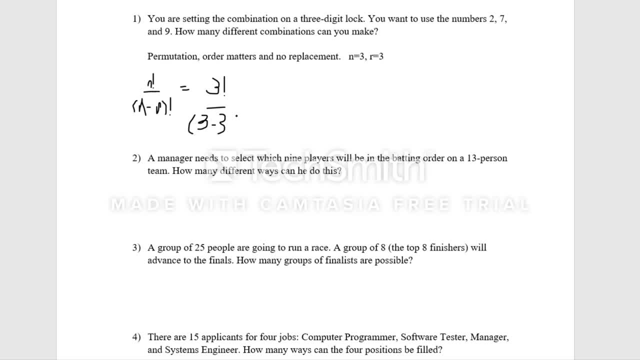 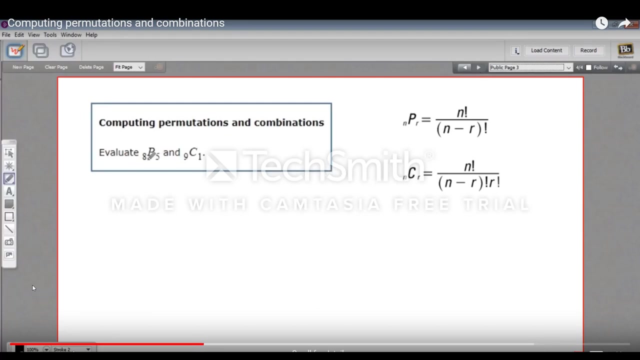 So what we're actually going to do here is- and in the next video we will learn how to solve problems using factorials. so this problem says evaluates 8 P 5 and 9 C 1. so what this means is we're asking how many permutations are there when you choose five things out of a group of? 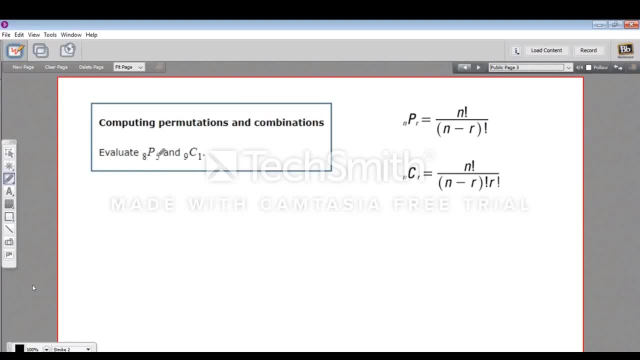 eight and that the order matters. to do this, you take the total number of things, that's our eight, and you take the factorial that and put it over the factorial of the total number minus the amount you're choosing. so this would mean in this case 8 factorial on top and on the bottom, n minus R, so 8 minus 5 it. 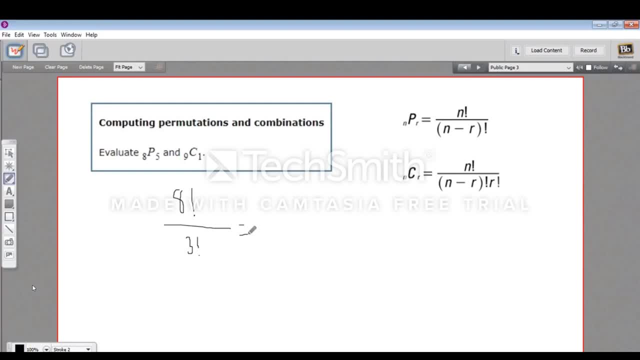 would be 3 factorial. when you're calculating these it's it's good to write them out until you get really used to it. maybe you can do some of this in your head. but 8 factorial is, of course, 8 times 7 times 6 times, 5 times, 4 times, 3 times 2 and. 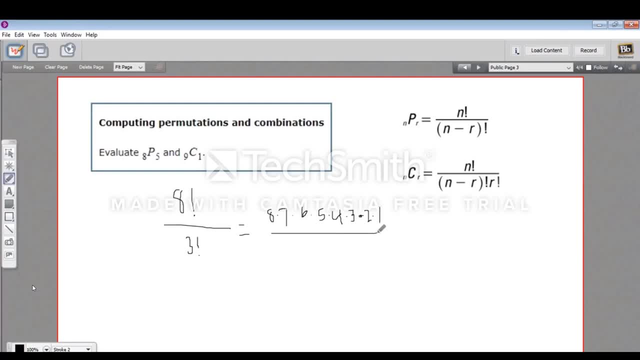 technically times 1, but you know the times 1 doesn't really change anything. and then 3- factorial- I'll write it down here- is 3 times 2 times 1. what you're gonna see is that this and this will cancel and you're gonna get a lot of cancellation with these permutations and 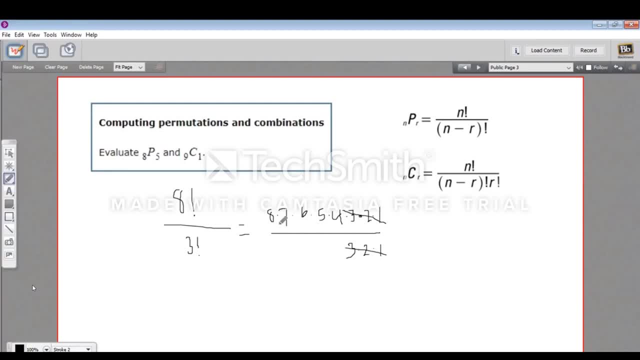 combinations, so be looking for that. so now we have 8 times 7 times 6 times 5 times 4, and at that point you'll probably want to get out your calculator: 8 times 7 times 6 times 5 times 4, and I am getting 6720. permutations tend to be: 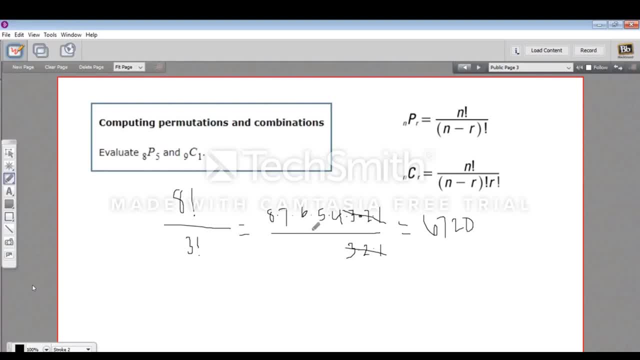 bigger, because when the order matters, there are a lot more ways to put things together. let's try this combination. you have nine things. you're gonna choose one thing out of that: 9. so in the combination formula the total number factorial goes on top, just like in the permutation, and on the bottom we have n minus R. 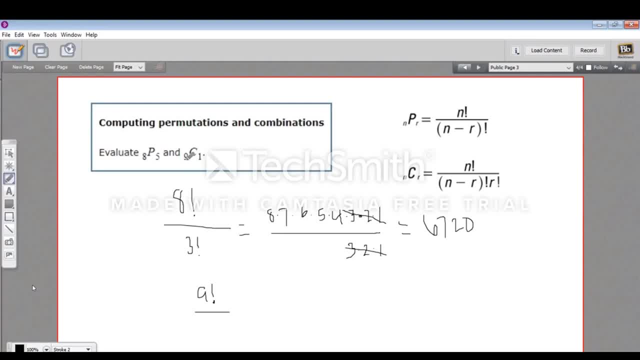 factorial times: R factorial. well, n minus R, 9 minus 1 is 8. so that's 8 factorial and R factorial. well, that's just one one factorial. that's not really going to change anything. Let's look at what we get when we do this one. We've